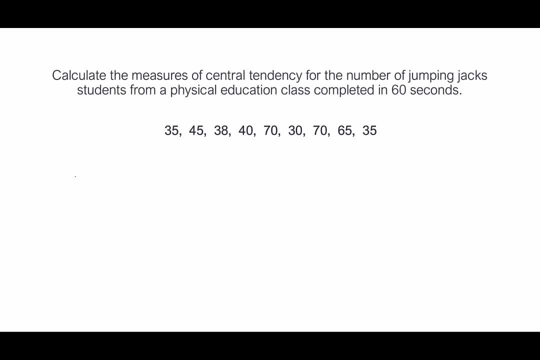 to add up all of these numbers, I suggest having a calculator. So if you need to pause the video to go get a calculator, do so now. Okay, you have your calculator. or are you going to do some mental math? Because mental 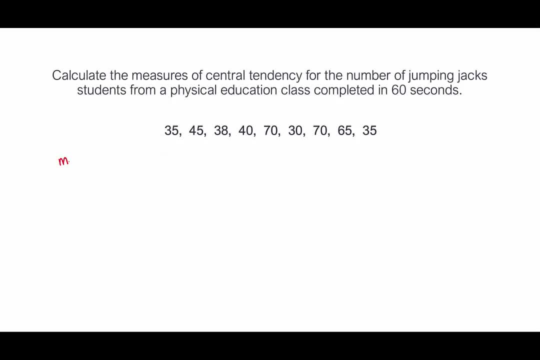 math is good too. Alright, to calculate the mean, we need to add up these numbers. So we have to add up 35 plus 45 plus 38.. 35 plus 38,, blah, blah, blah plus 35. When I added these all together, I ended up with 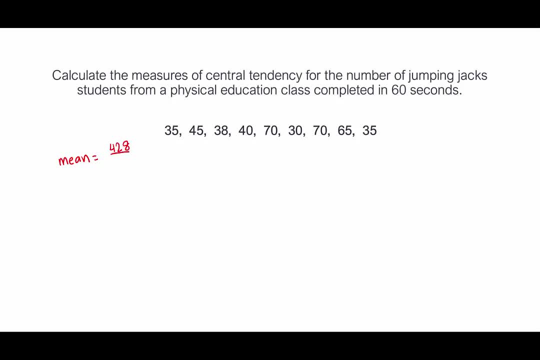 428.. And then we're going to divide by the number of numbers in the set. So how many numbers do we see? One, two, three, four, five, six, seven, eight, nine. This indicates there were nine students participating in the jumping jack, 60 second off. So we're going. 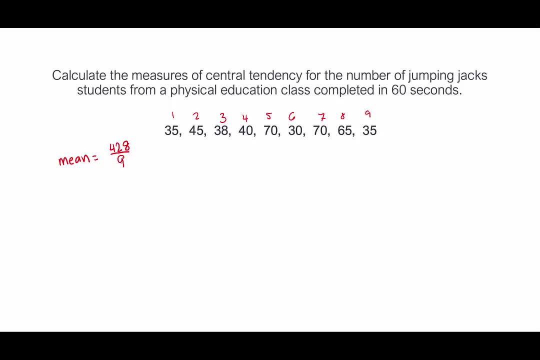 to divide by nine And when we do this we end up getting a decimal. I think it's like 47.5555555.. If you want to round to the nearest jumping jack, that probably makes sense, because we don't you know, even if you're in the middle of a jumping jack when the teacher 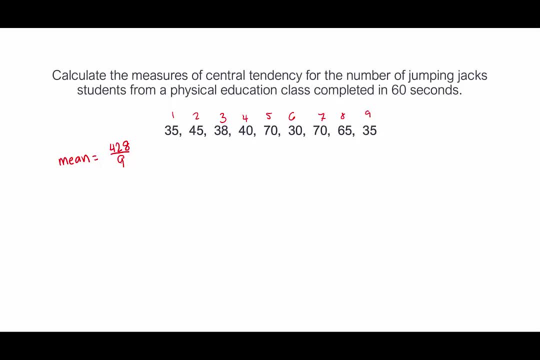 calls time. you don't count that as like. well, I was four tenths the way through it. No, we would either just not count it or round it up Because the five is in the tenths place. I'm going to bump it up and say the mean was 48 jumping jacks in 60 seconds. 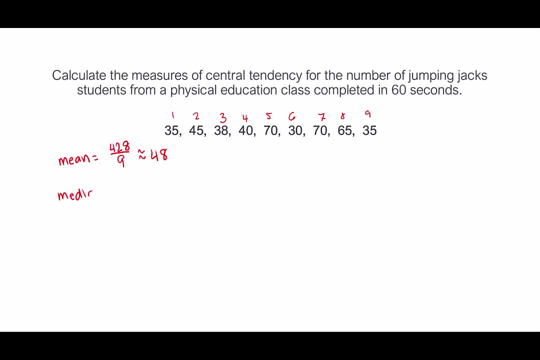 To calculate the median. we want to line up these nine numbers in order from least to greatest. Since there are nine numbers and nine is an odd number, I am expecting just one number in the middle. I'm going to start with that 30. And I'm going to cross it off as I go. 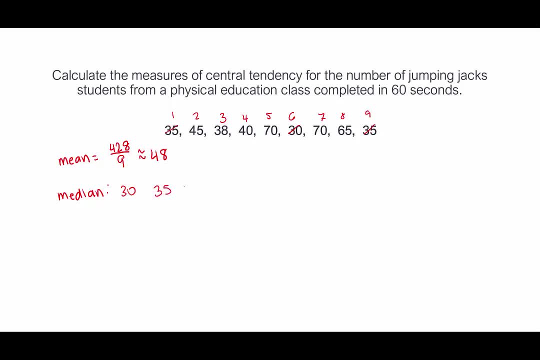 Then I have a 35 and a second 35. So already I know we at least have one mode. We have a 38,, 40,, 45,, 65, and two 70s, 65,, 70, and two 70s. 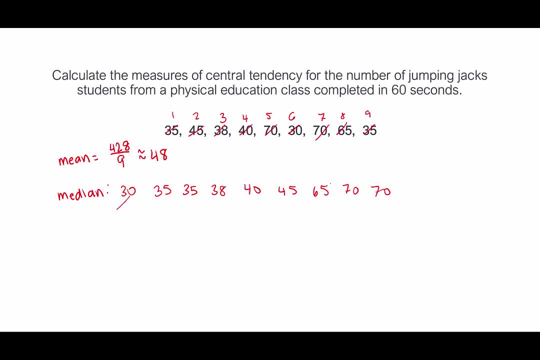 And 70.. Okay, so to calculate the median. I'm just going to cross these off, so it's not those Next extremes, Next, next, And I see 40 is right there in the middle. There's four on the left of it And four on the right of it. The median is 40.. Lastly, to calculate, 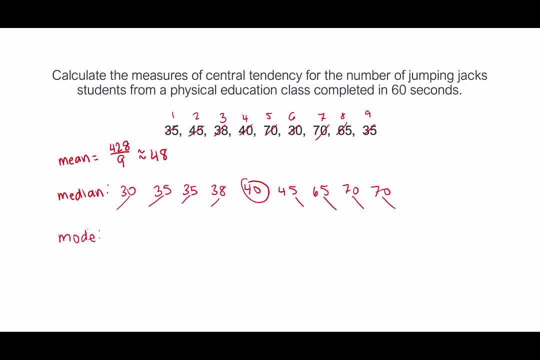 the mode did we see one or more numbers that repeated more than once? I remember writing 35 twice, right, That repeated twice And 70 repeated twice. So this one is bimodal. We have two modes of 35.. 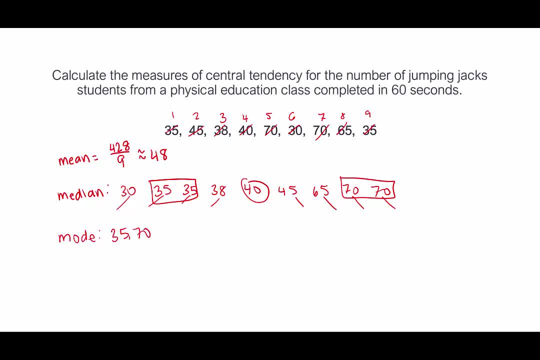 And 70. 70. So to summarize our data, I'm just going to go over here and just write everything all neat so I can just put a box around it. The mean we calculated to be about 48 jumping jacks in 60 seconds. The median we found was 40. And this was a bimodal. We have two modes of 35 and 70.. So that would be the measures of central tendency for this first example. So far, so good. Let's do another one. 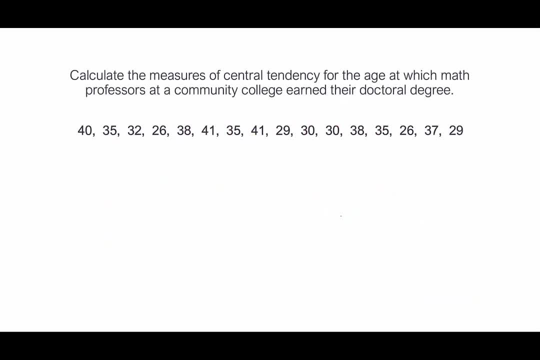 Here we want to calculate the measures of central tendency for the age at which math professors at a community college earned their doctoral degree. Again, I strongly suggest having a calculator out And we also want to make sure when we're calculating the mean. it's very easy when you're using a calculator to have a typo right, to put a two instead of a 29, or it's put 229 because you hit the button twice by accident. So we want to make sure when we're calculating the mean that it does make sense, right If I'm calculating the mean of these numbers and I somehow get 54,. 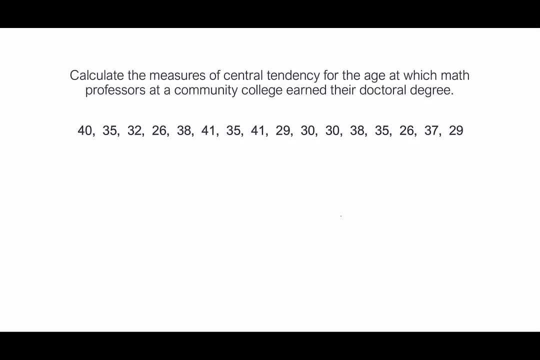 well, that's not good, because the largest number in my set isn't even 54. So that indicates to me that I made some sort of computational error. I might want to go back and check my work. So to calculate the mean, I'm going to add up all of these numbers. When I added up all these numbers, I ended up with 542.. And how many professors were there? Well, there was 2,. 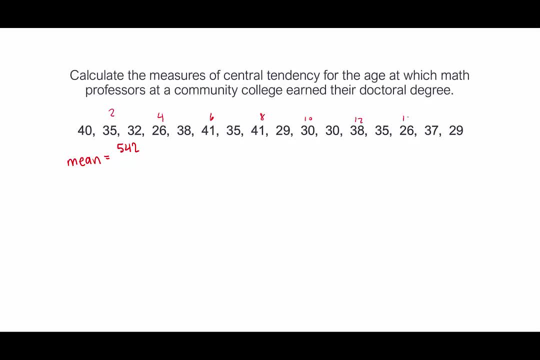 4,, 6,, 8,, 10,, 12,, 12,, 14,, a total of 16.. Aha, A total of sixteen. So I want to divide that down, each number, each number, by 16.. And again I'll round to the nearest year. I'm not going to do partial years here. 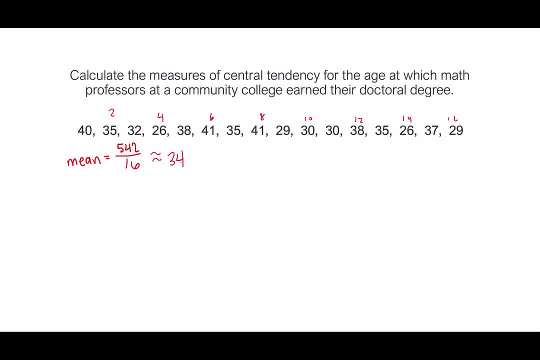 When I do this division, I end up with about 34.. So 34 years is about the mean for this data set. Next, we want to find the median. I'm going to need a lot of space for this because there are 16 values that I need to put in order, So I'm going to squish it all the way over there. 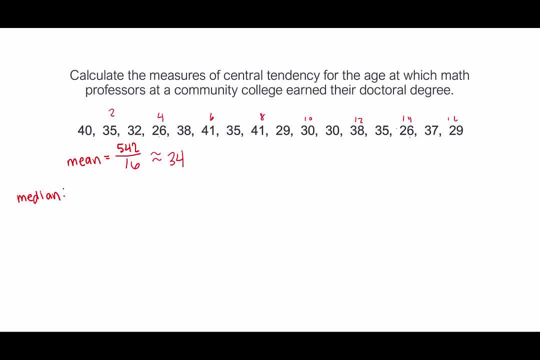 And let's start with the 20s. So I see a 26 and a 26 of 29.. Okay, so two 26s- 26,, 26,, 29, 29.. How about I'm going to cross those out so I don't use them again. Okay, now I see two 30s. 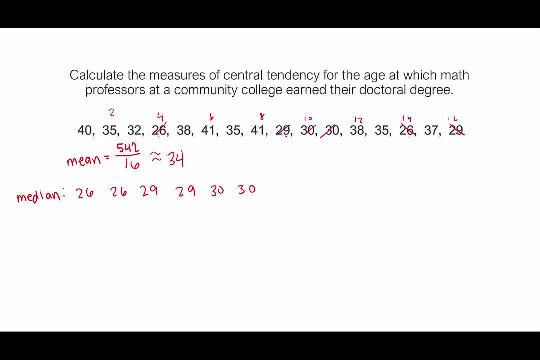 right there. So that's nice, They're right next to each other. A 32 right here, 32.. Then I have one, two, three, 35s, 35 and 35. Then there's two, 30.. Oh wait, wait, wait, There's a 37 before. 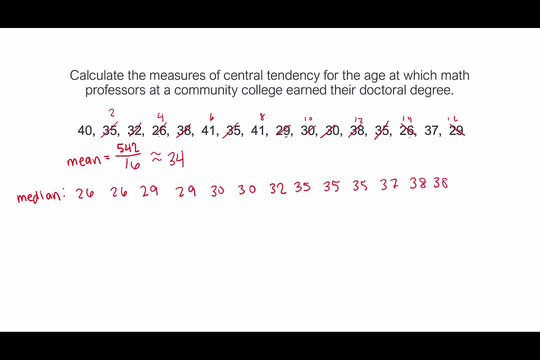 those two 38s. So one 37,, two 38s, 37,, 38,, 38. Then I have 40 and two 41s. Oh, I am going to get it to squish these all in, Okay. 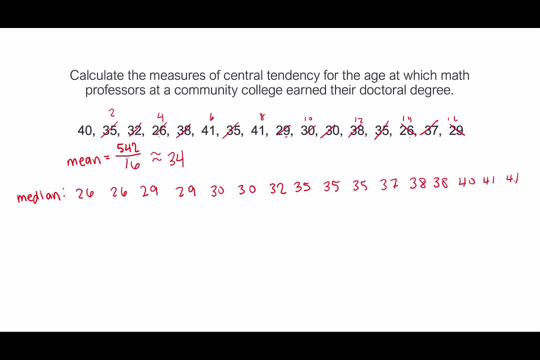 So there are all the numbers, Because there were a lot of them. I'm just going to double check that I really have 16 numbers here, So 1, 2, 3, 4,, 5,, 6,, 7,, 8,, 9, 10,, 11,, 12,, 13,, 14, 15.. Okay, 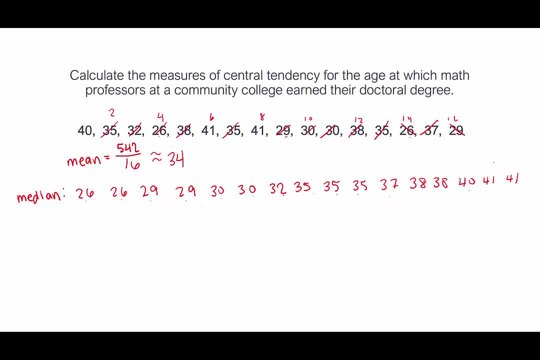 I did count 16.. So now I'm also expecting there to be two numbers in the middle. So if I do this calculator, if I go to calculate the median and there's only one number in the middle, I might have left a number out. So it's a nice. 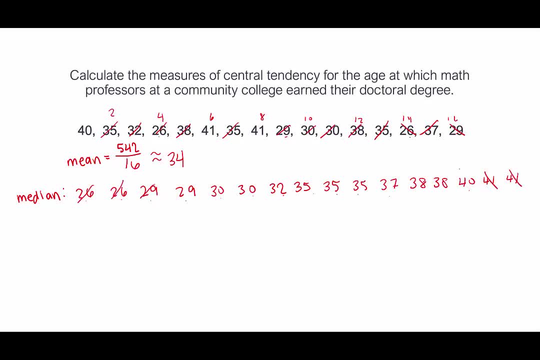 little check for us. I'm going to cross out: There's 3.. Here's 4,, 5,, 6, 7.. Aha, there are the two in the middle. They're 35s. I don't need to average them, I know the average of the same. 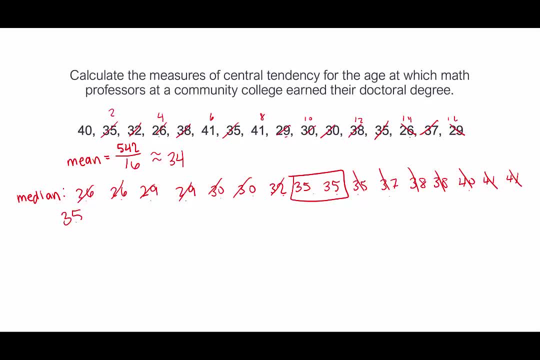 number is just going to be that number. So the median is 35.. Last, we want to look at the mode. So the mode is there one number that occurs more frequently than all the rest. There's two 26s, two 29s, but there are three 35s. 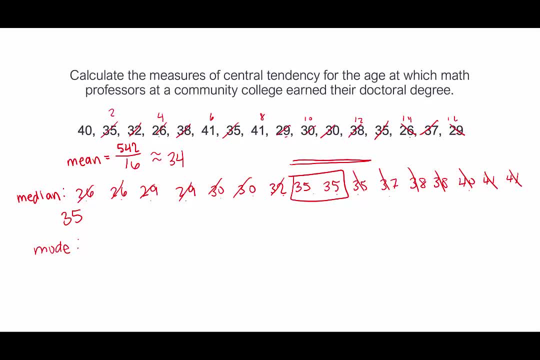 I don't think any other number repeats three times. So 35 is our only mode. This particular data set has one mode, and that one mode is 35.. These data values, these measures of central tendency, are much more compact than the previous example, aren't they? They're really close to each. 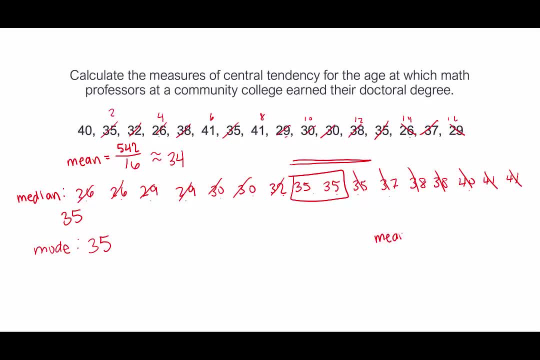 other. So just to rewrite everything: the mean for this particular set was 34, roughly. The median and the mode were both 35.. The median was 35. And the mode was 35.. Okay, Still good, We're going to do one more example, but this example is going to look a little bit. 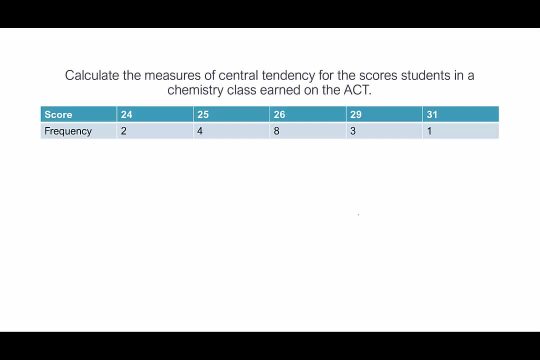 different than what we've seen in these past. two examples: I have it set up where I show the frequencies instead of writing all the numbers out. We can work with the frequencies or you can list all of the numbers. I'll show you how to use the frequencies because I trust that you can well. 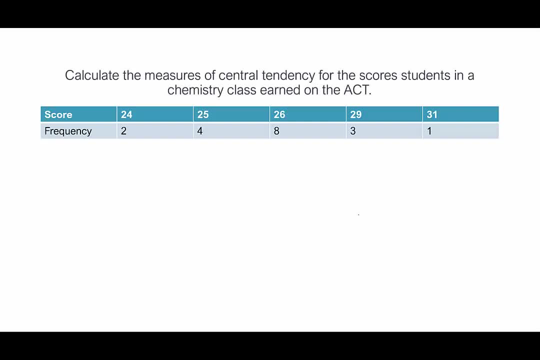 I'll talk about how you can line these up, But I'm going to show you how to use the frequencies, because I trust that you can well. I'll talk about how you can line these up, But I'm going to show you how to use the frequencies, because I trust that you can well. I'll talk about how you can line these numbers up, But let's see what we're looking at in this example. 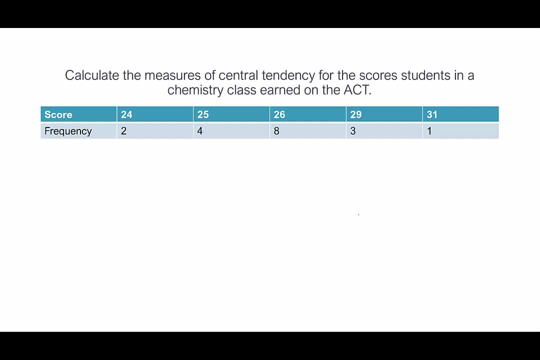 Calculate the measures of central tendency for the scores students in a chemistry class earned on their ACT. So we have five different scores and the frequency just means that many students scored that score. So two students got 24s, which means this would be 24 and 24, so that's representing two students. 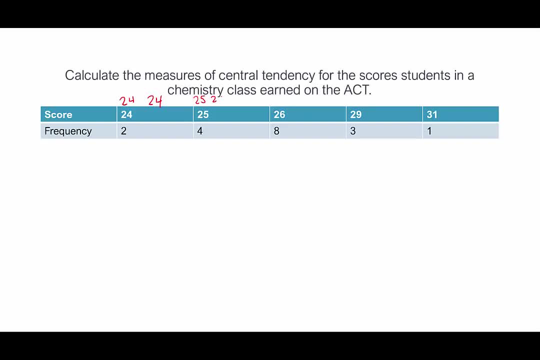 Four students scored a 25, so we would write 25 four times. Four students scored a 25, so we would write 25 four times. Four students scored a 25, so we would write 25 four times. You see what I'm doing here. 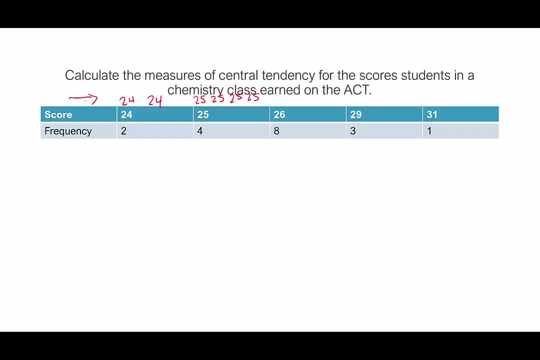 This would be listing it out if you want to list it out, but I'm going to use the frequencies instead. Feel free to list it out if you're more comfortable. I'm just super lazy and I don't feel like listing out 26 eight times. 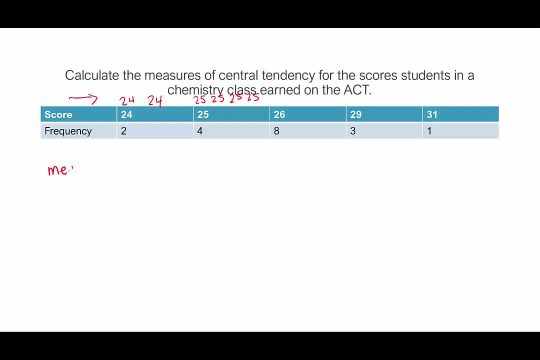 To calculate the mean, what we need to do is add up all of the values In your calculator. you can do 24 plus 24 and 425, so 25 plus 25 plus 25 plus 25 and 826s. Or because these numbers repeat, and repeated addition is multiplication, we could calculate: 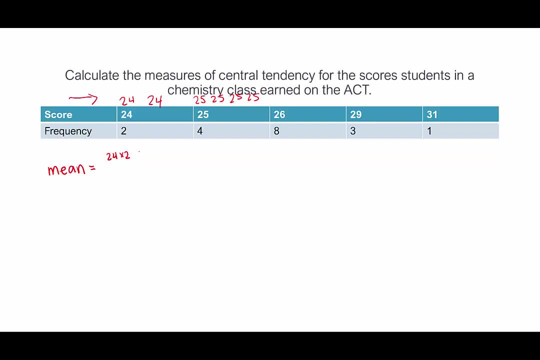 the mean by saying it's going to be 24, two times plus 25, four times plus 26, eight times plus 29, three times. Then I can just do 31, since there's only one. If you want to do 31 times one, that's fine. 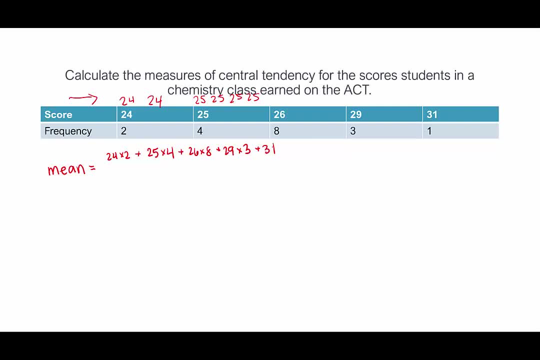 You see what I did there. Instead of doing each addition separately, I used the fact that multiplication is repeated addition to simplify this a little bit, or at least to make it shorter. Now, what am I dividing by How many students were in this chemistry class? 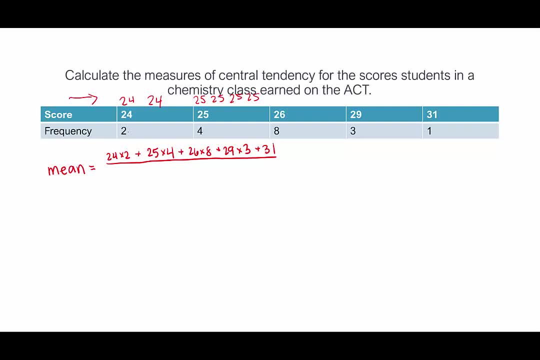 That would be the total in the frequency We want. to add up the frequencies Two plus four plus eight plus three plus one, That's a total of 18.. This particular class has 18 students in it. What I should see up here is, if I look at the frequencies, that should also add up to: 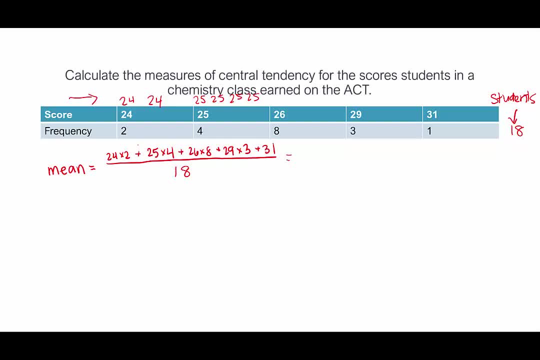 18, which it does. When we do this addition and multiplication, we end up with 474.. 474 divided by 18 gives us- and again I'm going to round, because the ACT is only measured in units- We end up with 26.. 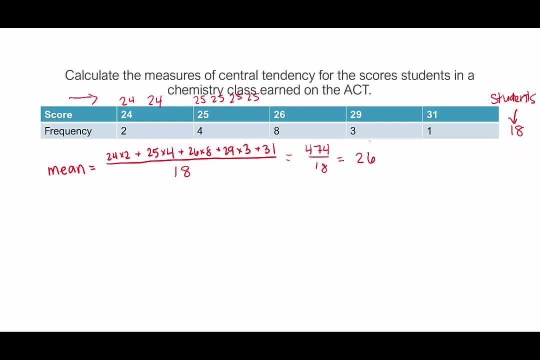 26 makes a lot of sense. 26 makes sense right, because the scores for the ACT were 24,, 25,, 26,, 29, and 31. So it makes sense that the mean would be 26.. How we doing. 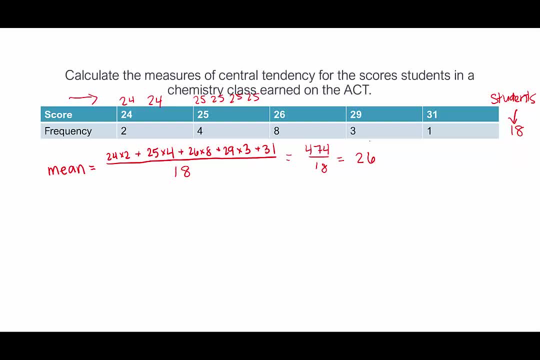 You okay, You're doing great, Okay. Next, to calculate the median. and again, rather than putting everything in order, I'm going to use the frequencies to help me. So one thing I mentioned in the video on medians is that if you want to find the median, you 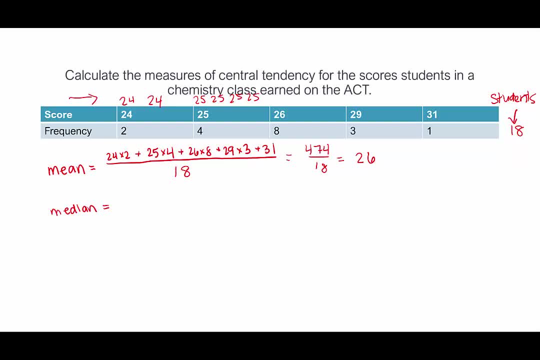 can actually use a formula In this case. we know there are 18 students, so we know we're actually going to have to add two values and divide by 2.. But where will those two values be? If there's 18 students, then the two median values will be found in the 18 divided by. 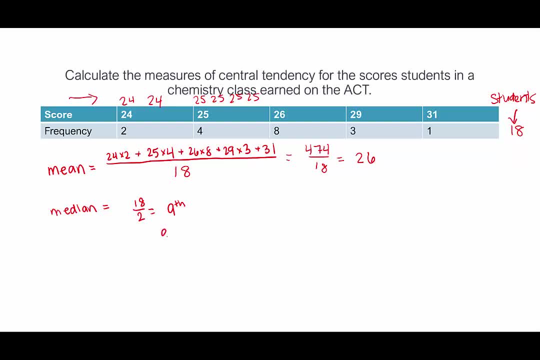 2 position, so the 9th position, and then 9 plus 1, the 10th position. So where are we finding this 9th and 10th number? And here's where this can get a little well, as if it wasn't already weird, it can get. 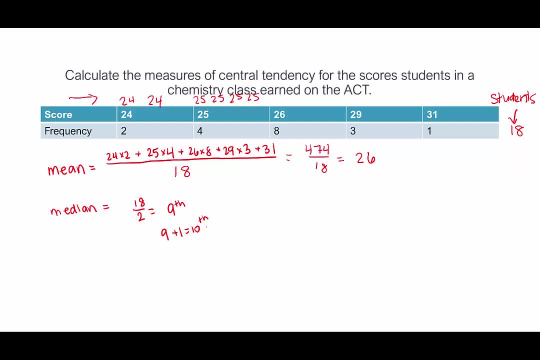 a little weird here. So to calculate, to find where the 9th and 10th students are, when we put these numbers in order, remember that there are 2 with 24 and there are 4 with 25.. So far we have 1,, 2,, 3,, 4, 5, 6 students accounted for.